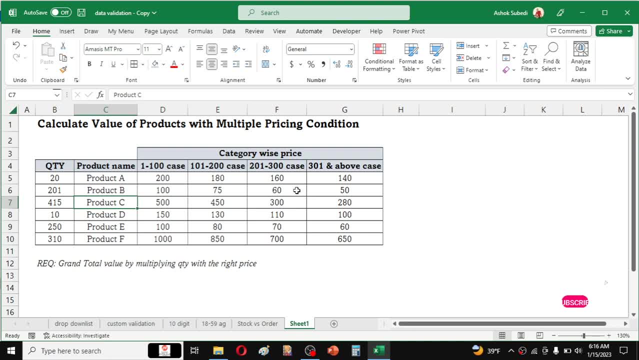 it will automatically multiply with the appropriate price. so to do this, here we need to add a one helper column and the column name will be this: here: here we have to write the price column- price for the product or price for the quantity- so this helper column will capture the appropriate pricing from this. 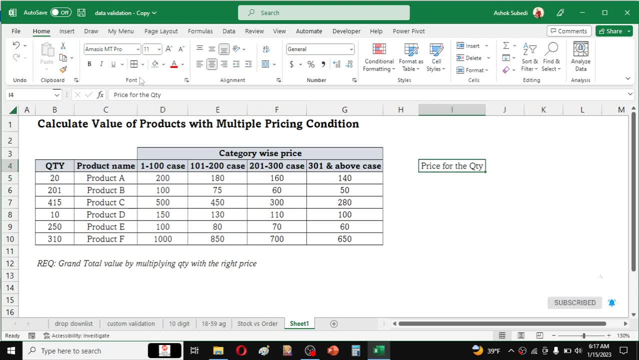 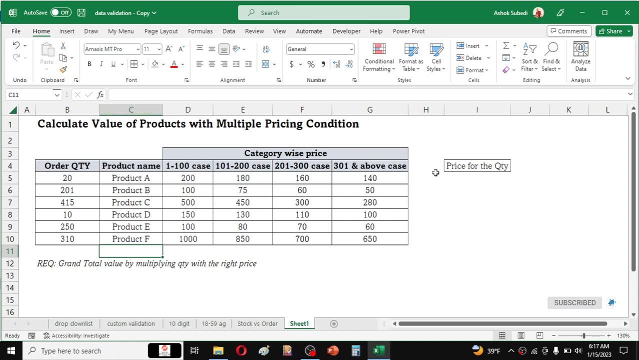 details. so here we have to use this formula to get the appropriate price for the quantity that we mentioned here. here i am making this order quantity, order quantity, and here, in this case we can use the ifs function equal to, then type ifs, ifs function, then open the bracket, and here we need to define the first logic. 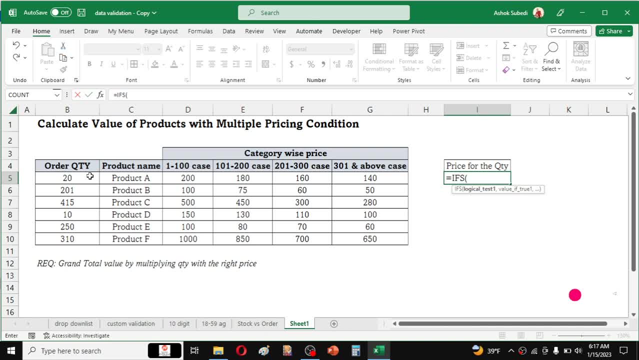 and our first logic is: if the quantity is less than or equal to 100. so here click on the quantity, then type less than or equal to sign, then click on this less than and equal to, then type 100. here, because the first condition is: is less than or equal to 100, now give a comma and here in this value, if true, we have to click on. 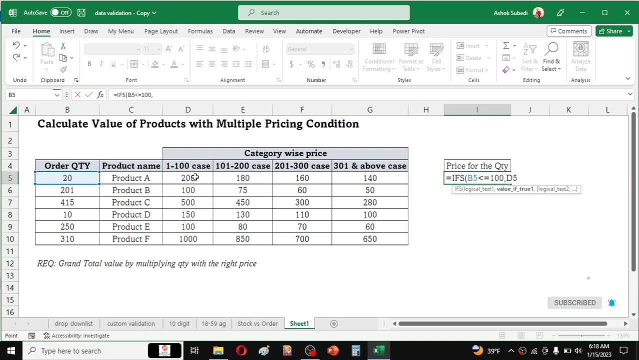 this pricing. click on the price which is given here. now give a comma. then we have to define the second logic, or logic number two, or logical test two. and this is: if this quantity is less than or equal to 200 cases, then give a comma. in that case our pricing will be this: 180. so click on 180. 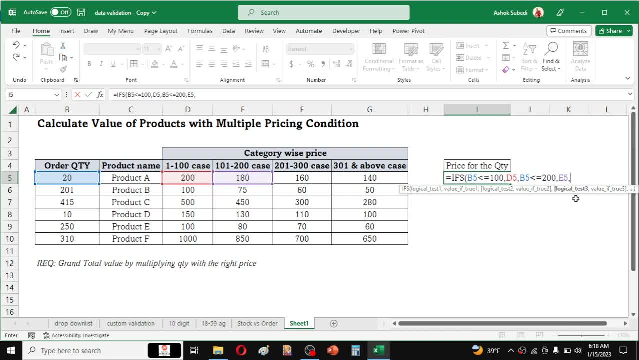 now give a comma. in this logical test three, we have to check whether this quantity is less than or equal to 300, 300. now give a comma. if the quantity is less than or equal to 300, then we have to define the second logic, or logic number two, or logical test three. and here in this: 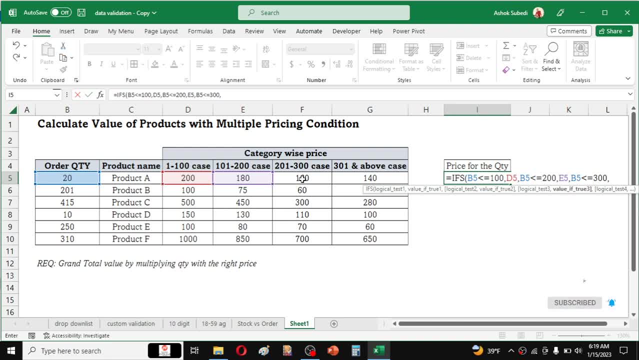 we have to select this price, which is 160. so click on 160. now give a comma. the fourth logic is if this quantity is greater than 300, because this is our last logic- when the quantity is 300 case and above, then our price will be from this G column. so here write this logic: if the quantity 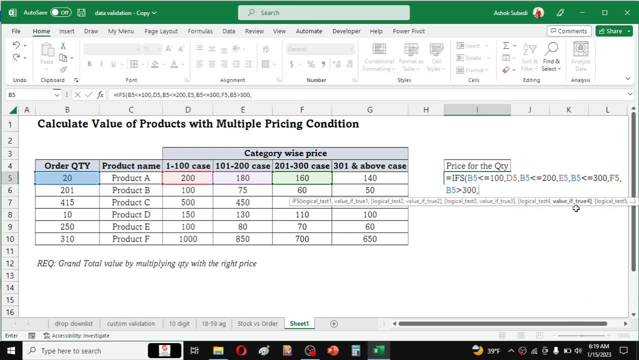 is less than or equal to 300, then we have to check whether this quantity is less than or equal to 300. then give a comma and the value if true, or the pricing will be this: 140. so click on 140 now close the bracket and hit enter now. here you can see the appropriate price according to the category. 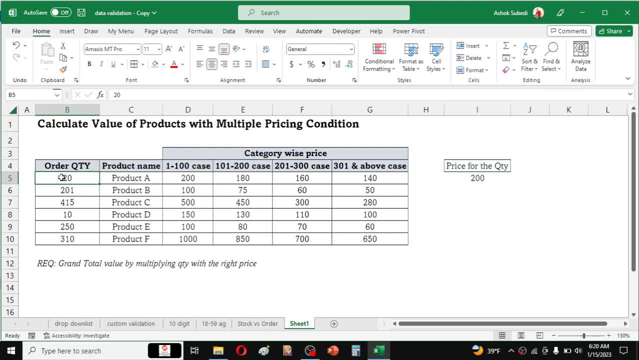 defined here is captured. here you can see the quantity is 20 units and the price is 200, which is captured from here. if the quantity is 1 to 100 case, then the price will be 200, and here you can see the price is 200 and here you can see the price is 200 and here you can see the price is 200. and. 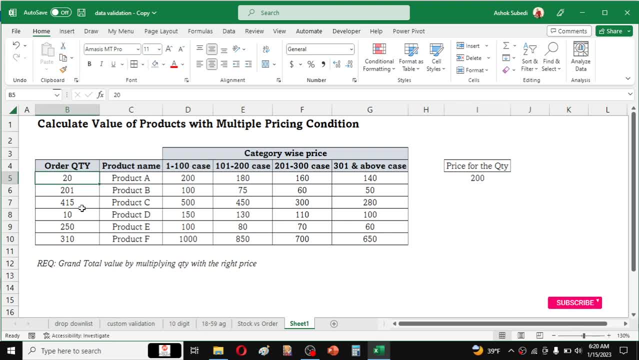 captured. for example, if I make this quantity or if I change this quantity to 450- here you can see the price is calculated as 140, because if the quantity is greater than 300 units, 300 cases- then the applicable price is 140. that's why the formula is displaying 140 here. similarly, if I make these: 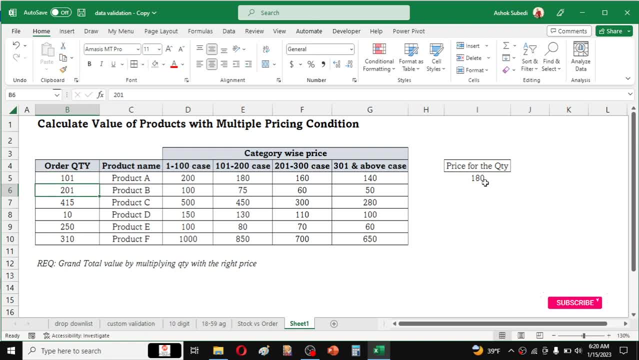 100 one case. then the price is calculated 180, which is calculated as 140. and here you can see from here: similarly, if I make these 200 and 90, in that case it is 160. so the price is calculating correctly. now you can simply drag this formula for your other products. just go here in the plus. 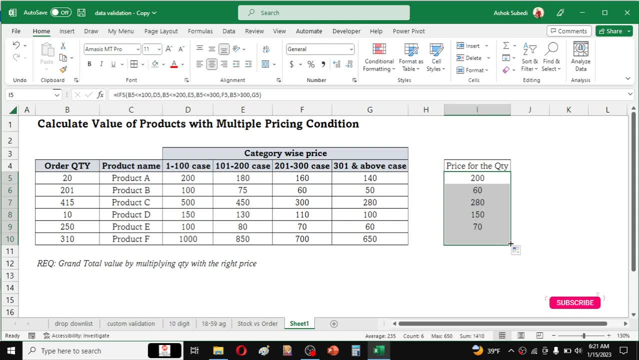 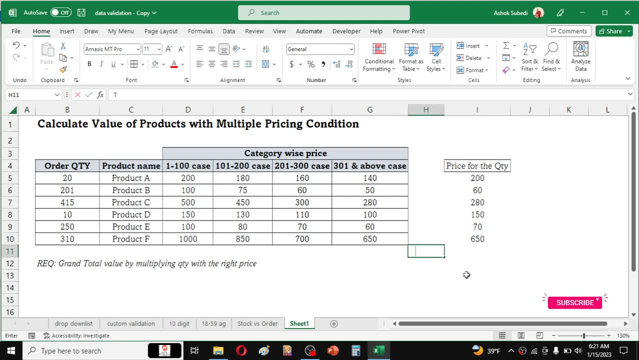 have filled here now to calculate the value of the quantity we have filled here now to calculate the. here we need to use this formula. here i am writing total value, total value, and the formula here in this total value will be. here i am writing the formula to calculate the total value, which is: 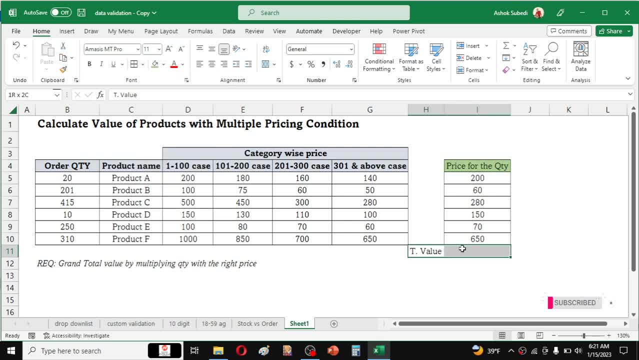 the sum product formula here in this total value. i am going to use the sum product formula, so click on this total sale where you want to calculate the value. now press equal to. then type the sum product function here- sum product- then open the bracket. now, here in this array, one we need to: 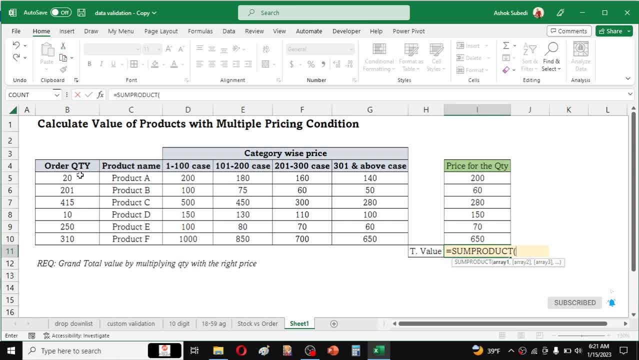 select the quantity range from here. in this way, the quantity is selected. now give a comma and in this array two we have to select the price range which we have just calculated here. so select this range of price in this way. now close bracket and hit enter, and here you get. 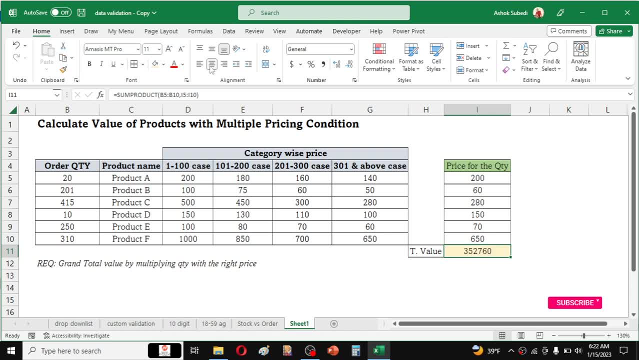 the total value for the products or total value for the quantity that you defined in column number b. so this is the total price for these quantities and this is now automatically calculated. after developing this, we have to only change the quantity here or a quantity here, and all the values will be. 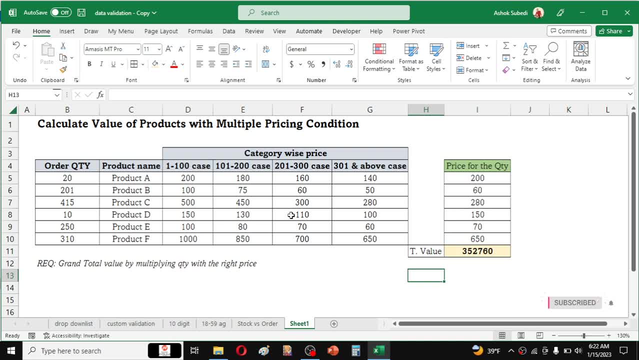 calculated according to the pricing category. now, for example, if i delete this from here, delete, the value is now zero and here the price is displayed. and this, this is displayed because we don't have defined any quantity here. so even if there is no quantity, then it will not impact anything in the value. 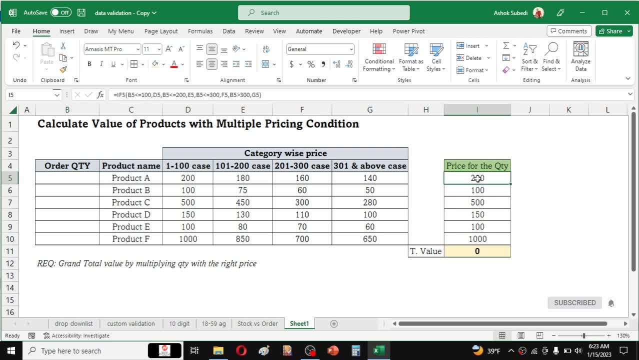 because the zero quantity multiplied with the price will be zero. that's why if some quantity is blank, then you don't have to worry, because if, for example, if i put here some quantities and if i leave one product blank, in this case this value will not be wrong, because if there is zero,